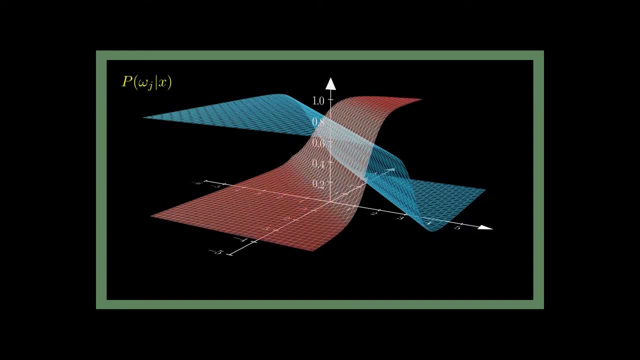 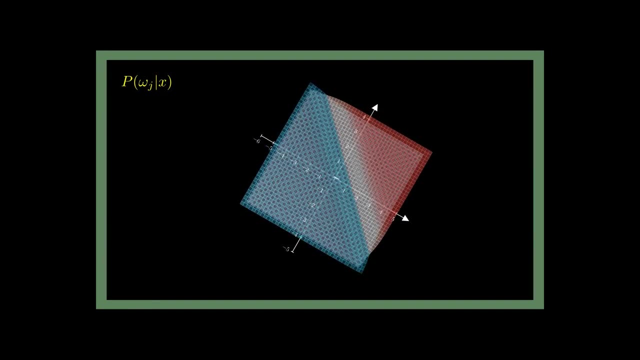 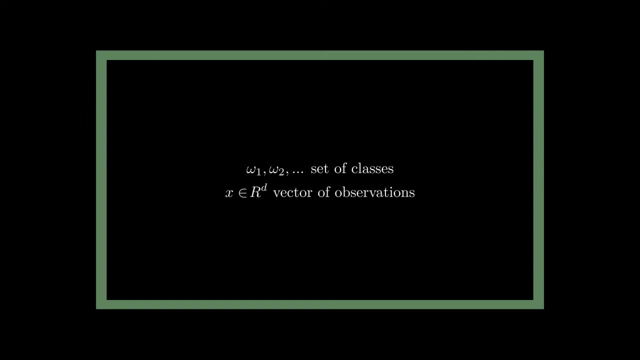 we can construct a optimal classifier under the assumption that we have full knowledge about the data generating process and probability distributions. I highly recommend watching the video to be more familiar with the notations, what which probability means and how the classifier works. But in this video we will loosen the assumption of full knowledge and try to learn. 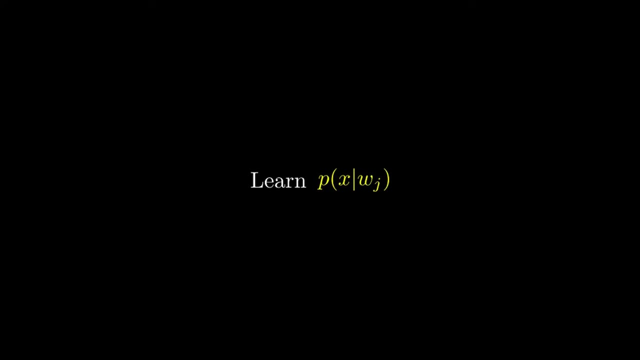 the distribution p of x, given omega j from our data. So, to stay true to our previous example, we would catch fish and measure their selected features. But for today's visualization we will stay in one dimensional space. Now we would have a lot of feature vectors or values for each class, for example the salmon. 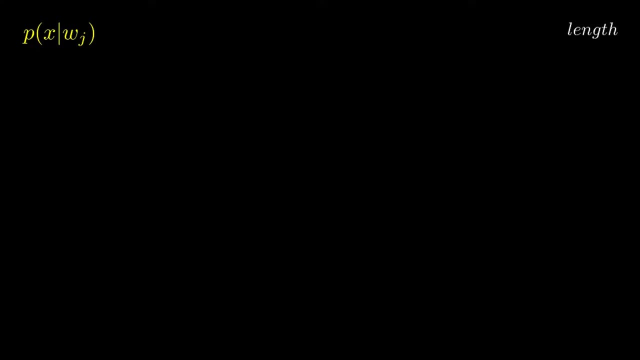 From that data. how do we build or learn the likelihood? Well, we could simply build a grid in input space and, for each class, build a histogram that counts the number of observations that belong to each bin. But many bins will have zero observations, not because the data probability is truly zero. 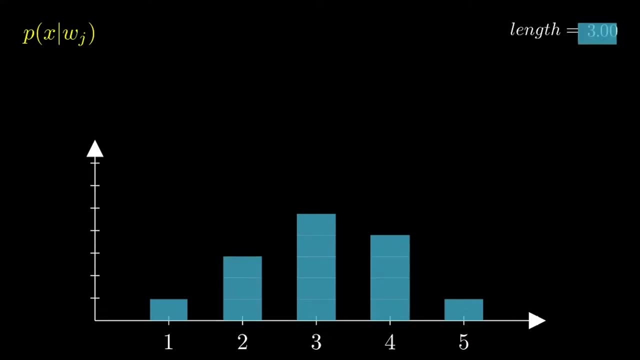 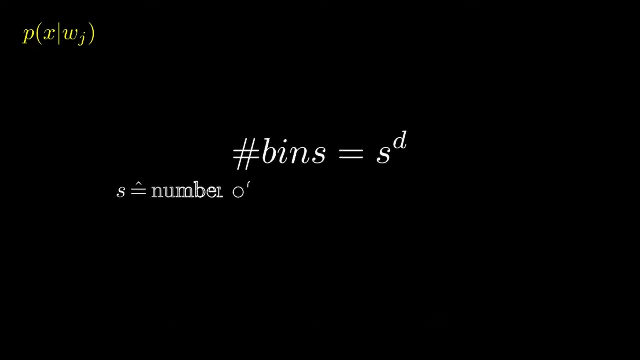 but because only finitely many examples have been observed. But, most importantly, the number of bins is s to the power of d, where s is the number of steps along each dimension and d is the number of dimensions. So it rises exponentially, which is very bad, since such data can easily have a large number of dimensions. 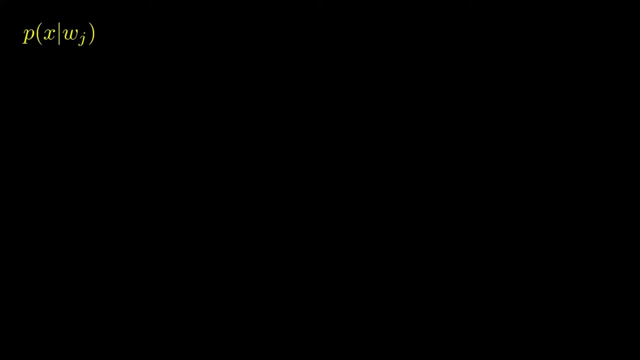 What can we do now? Well, another idea is a model based approach. The idea here is to assume that p of x, given omega j, is a non-parametric form, for example a Gaussian distribution with a mean mu j and covariance matrix, sigma j. 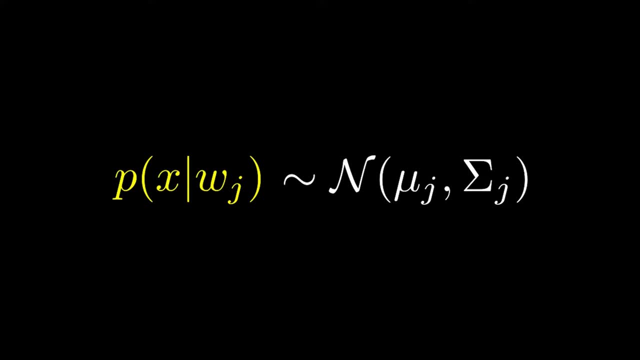 Where mu j and sigma j are the parameters of the distribution. So the goal now is to estimate, or in other words learn, the parameters of the distribution so that it best fits the few observations we have. With this model-based approach, we only need to learn a finite and typically small number of model parameters, and not the whole. 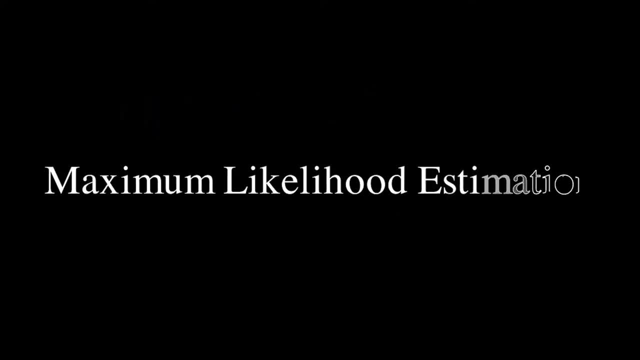 data distribution. One such approach is maximum likelihood estimation. We assume we have a data set d of our observation vectors x1, x2 up to xn. Each xk has d dimensions and has been generated independently and from the same density function p of x. given theta, Theta hereby is just the. 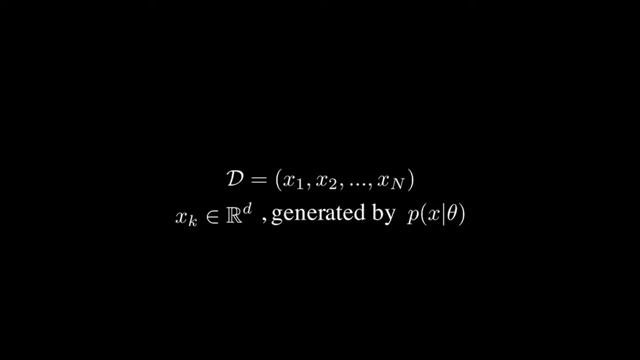 variable for all parameters of the distribution. This will hopefully make more sense in a bit. So if we look at each xk independently, we can assign a probability distribution, for example a Gaussian, to each one data point we have and try to find a theta that best represents the data. 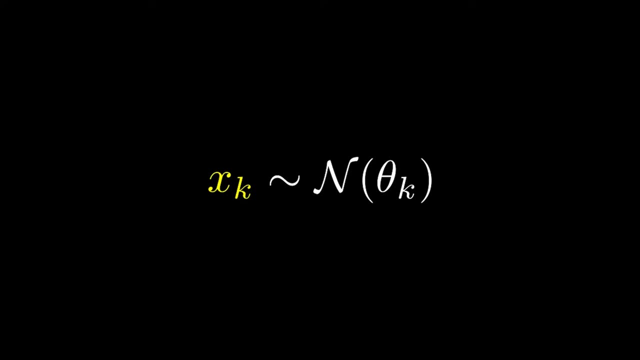 If we stay in one-dimensional space with a Gaussian distribution, we only have one parameter, the mean, which is just our theta. It's just a more general naming convention, Continuing. if we only look at an observation of, for example, x1 is equal to minus 0.5,. 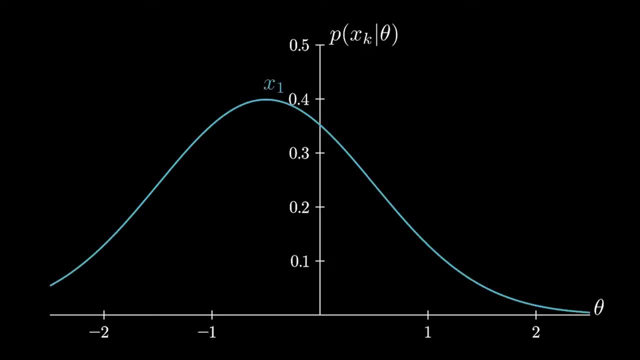 the mean of the distribution is exactly this minus 0.5.. Again, we are looking for a parameter theta that best represents the data we observe, Since we only have one observation, namely x1 is equal to minus 0.5,, choosing a theta or just the mean of the distribution, 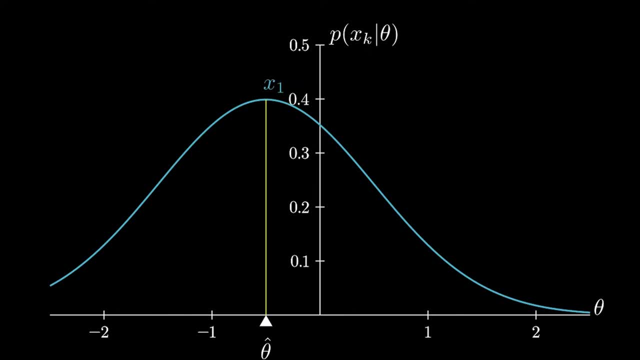 that corresponds to this value will provide the optimal result. Now we have, for each of those data points, independent Gaussians with a respective mean or theta. To make this more clear, the real objective is to find the theta for our Gaussian that best represents our whole data. So we want to look at the joint density function. 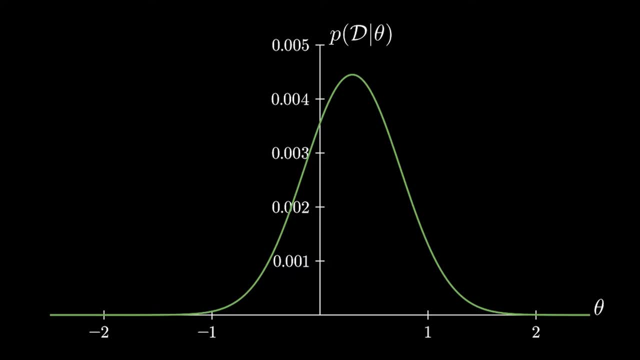 or also called the likelihood of theta, with regards to the whole data set D, which can be simply written as the product of all the independent density functions, We now have one density function over the parameter we are looking for and the best theta is given by the argmax for theta of the joint density function. 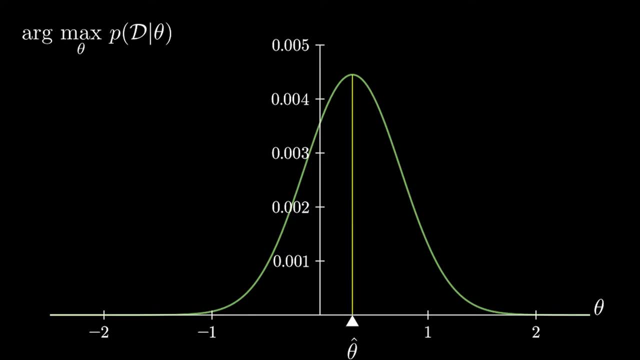 So intuitively, just the theta with the highest probability. But we of course also need to determine that analytically. And how do we find the maximum of a function analytically? Exactly, we need to find the theta that sets the derivative. 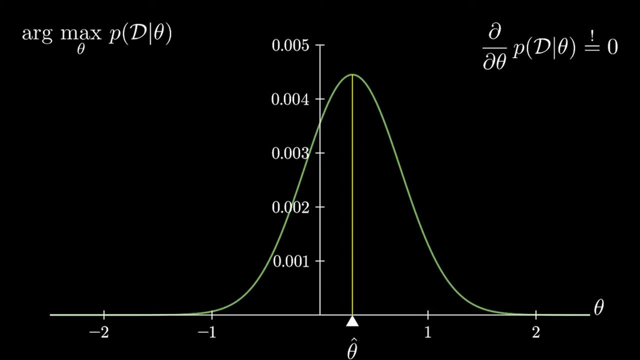 or, in a multivariate case, the gradient of the function to zero. But to be able to do this analysis the function has to be concave, meaning if you select two points on this function and connect them through a line, the function between those two points continues above the drawn line. This has to be valid for all points. 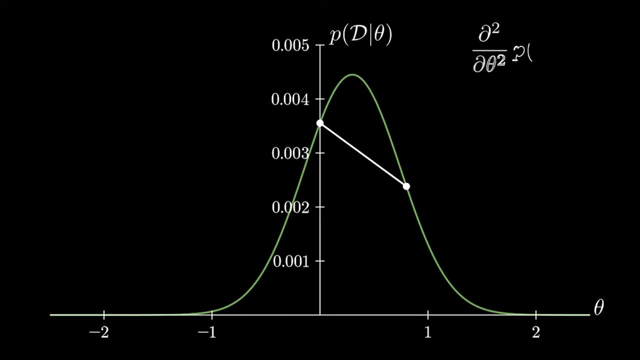 you select, Or analytically. the second derivative has to be zero. Now, as you can see in our example, this is not the case. The function p of d, given theta, is not concave. So the idea is to transform the function in a way such that it doesn't change. 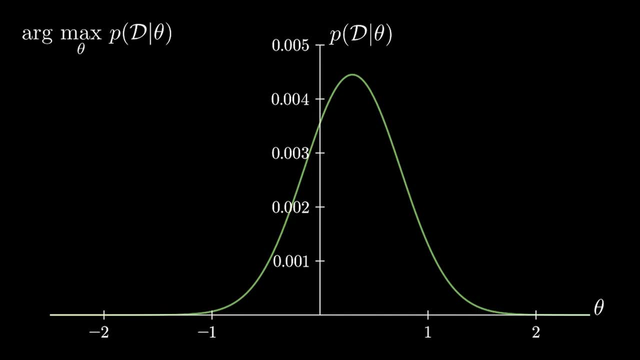 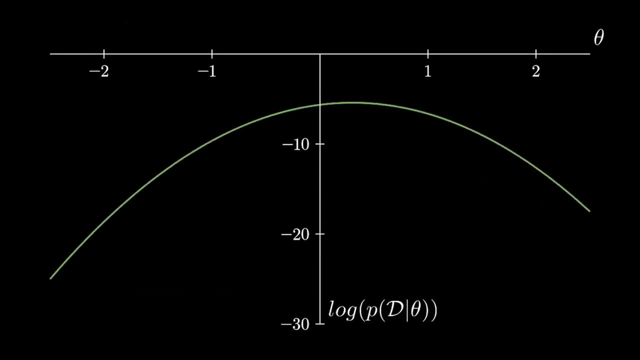 the outcome of the argmax and it makes the function concave. If you have watched the previous video on Bayes decision theory, you know that applying the logarithm function ensures those two properties mentioned. Ok, since we now have an intuitive understanding of what the objective is. 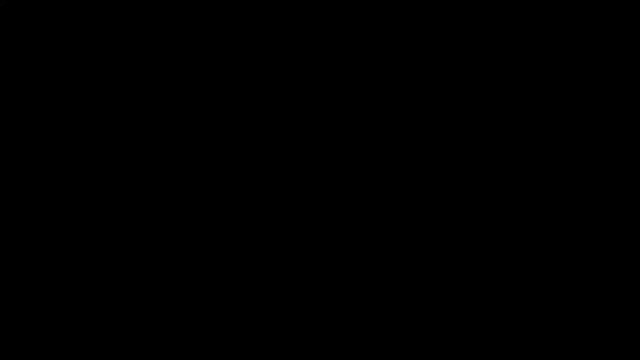 and how we want to solve this problem analytically. let's finish the example of one-dimensional data for a Gaussian model. We have already derived that the objective function p of d, given theta, is the product of the independent density functions, which are all gaussian. 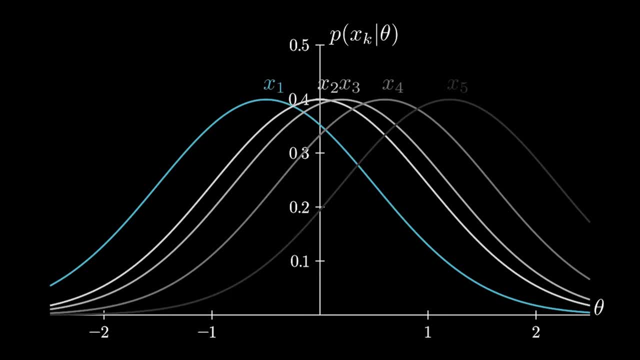 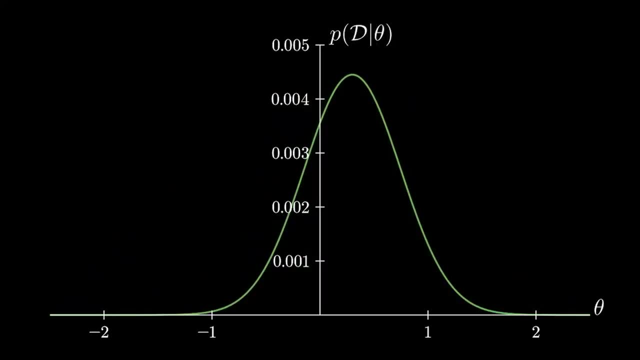 Each Gaussian hereby has their own theta as the mean, but we're looking for the theta that best represents the whole dataset d? Intuitively we know that it again has to be the mean of the new joint density function, or just the theta with the highest probability To determine that analytically. 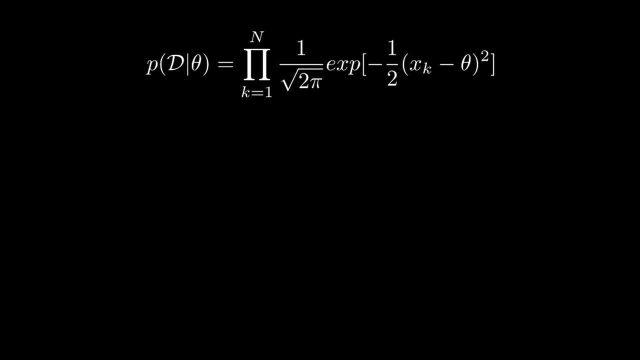 we have to transform our objective function into a concave one without changing the outcome of the argmax. So we apply the following method: logarithm. Now the logarithm of a product is just the sum of the logarithms. Now the log of the 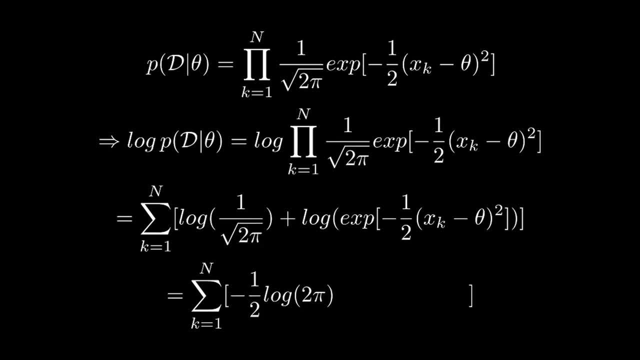 first term is minus one half times log of two pi. since one over square root of two pi can be written as two pi to the power of minus one half, Then the log of the exponential is just the identity function, so it simply removes this exponential. From here on we want to find the one theta, so that 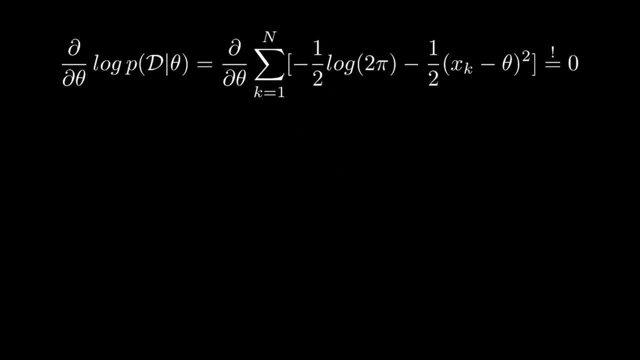 the gradient of the log of p of d, given theta, becomes zero. If we use the simple rules of building the derivative, we get this result. We can now do some equivalence transformations and get to the point we already intuitively suspected: The optimal theta, that the maximum likelihood 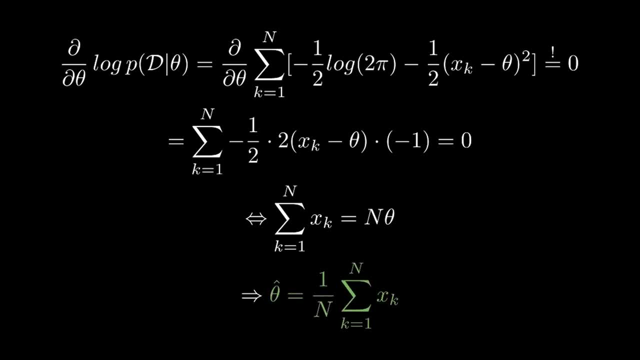 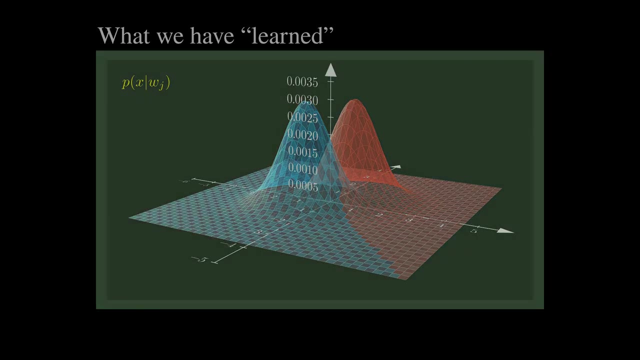 estimator gives you is the mean of the whole data, And this also holds for multivariate gaussians. To now build the classifier we have discussed in the videos on Bayes decision theory, we need to go through this parameter estimation process for each class that we have. 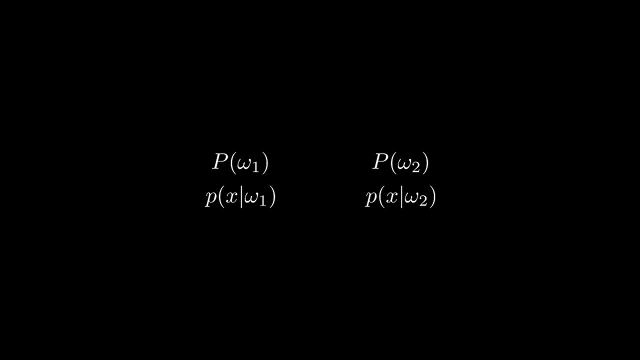 Then we finally have all the information about the probability distributions we need. We have, for example, caught a lot of fish and could determine the prior distribution, or we simply assume to know it, And through the features of those fish we can estimate or learn the respective likelihoods. 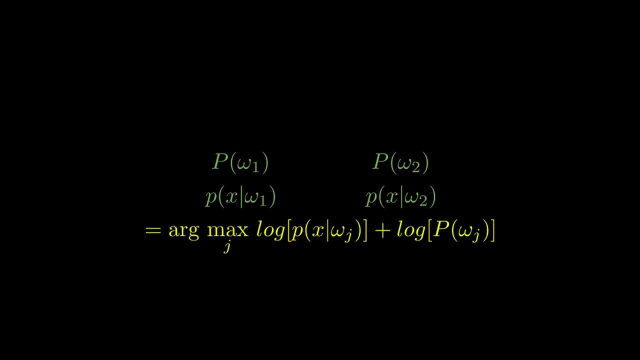 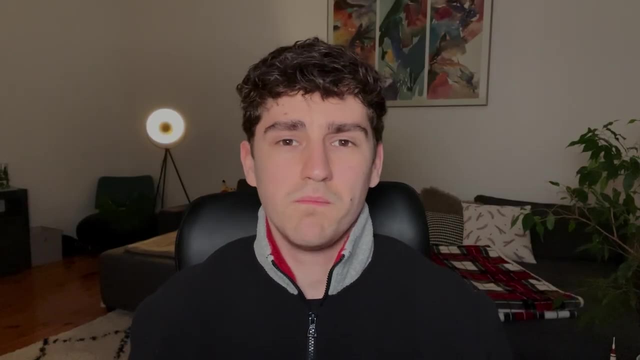 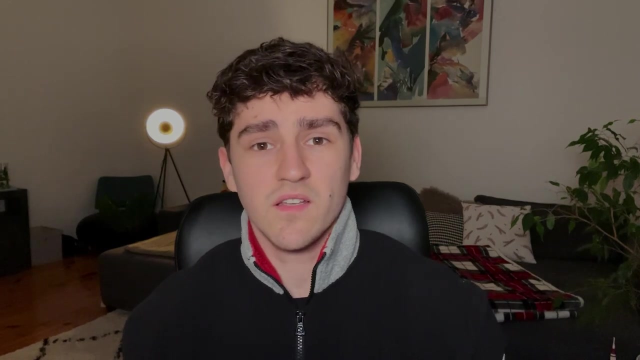 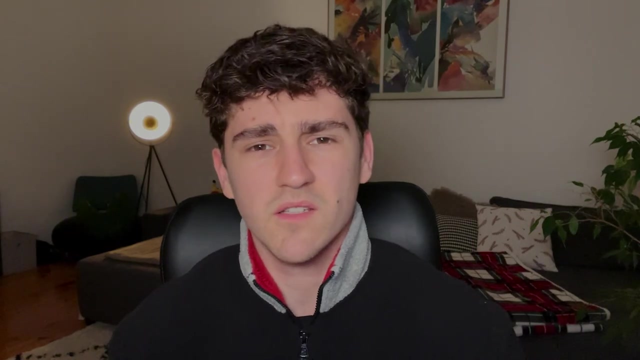 Finally, we apply the optimal decision function given by Bayes decision theory. Okay, guys, that was it for today. There is another Bayesian parameter estimation approach which is more difficult, also computationally, but provides a confidence estimation Nevertheless. I think that this maximum likelihood estimation approach is well established and better to 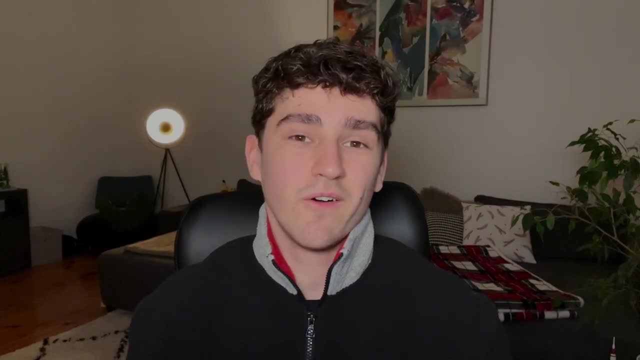 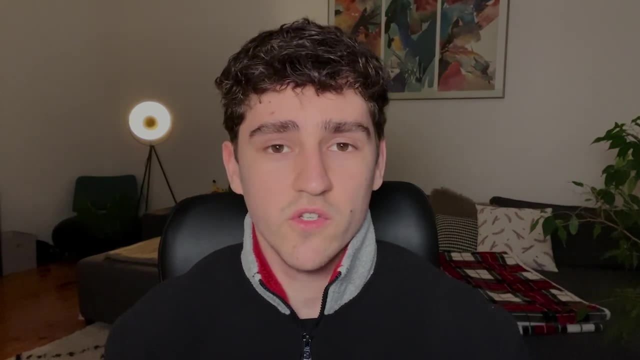 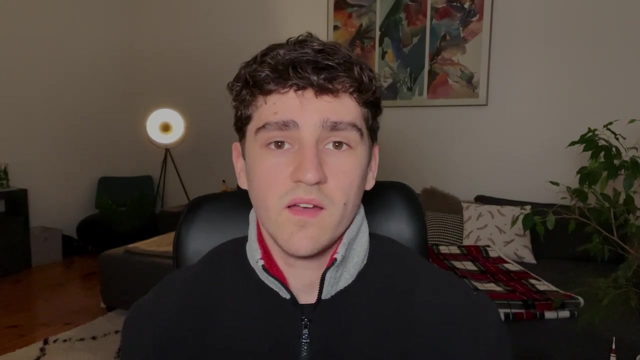 understand. If you really want me to make a video on Bayesian parameter estimation, feel free to leave a comment below. In the next video we'll be looking at classification approaches that need even less information, For example, only the means of the data distributions or the means and the covariance matrices between the class distributions. 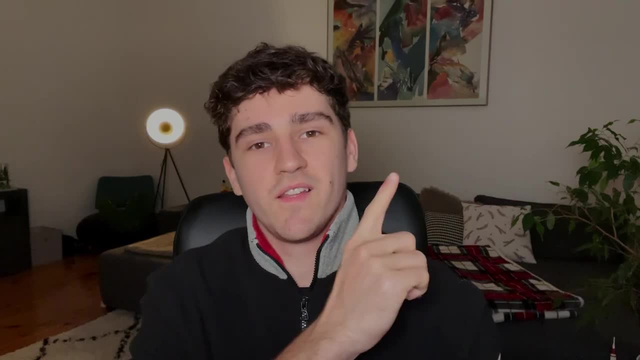 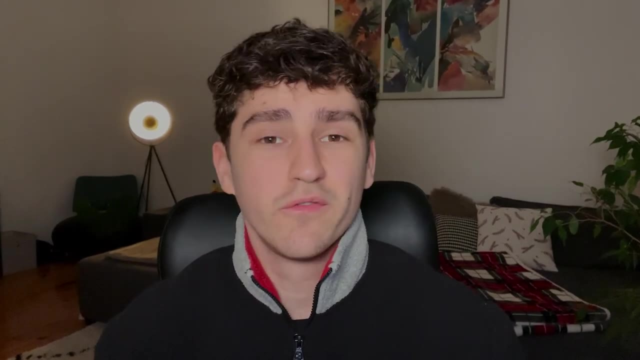 I will have all my machine learning videos in a playlist that you can click up here. I really hope you have enjoyed this video, found it helpful and learned something new, And if so, don't forget to leave a like and subscribe. I really hope you enjoy this kind of more theoretical. 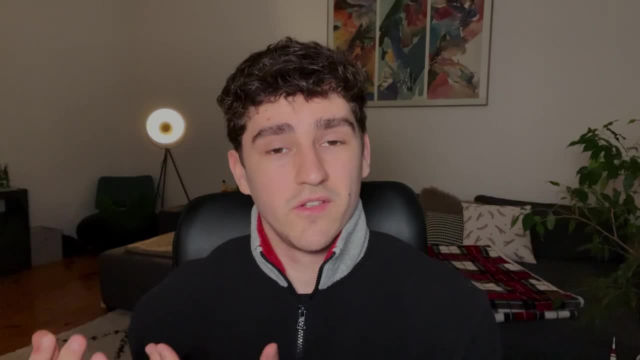 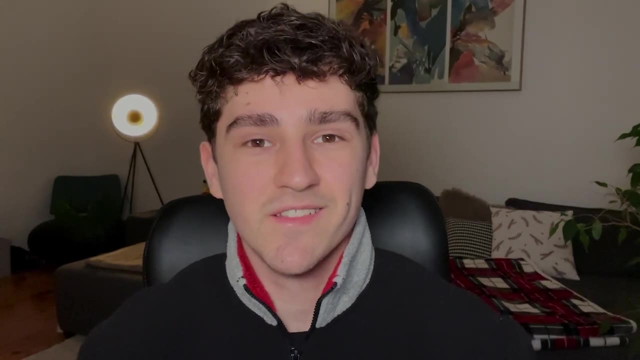 content, or if you don't look at my other videos that are more relaxed or are more about the uni life itself. And with that said, as always, thank you very much for watching and I will see you guys in the next one. Bye.